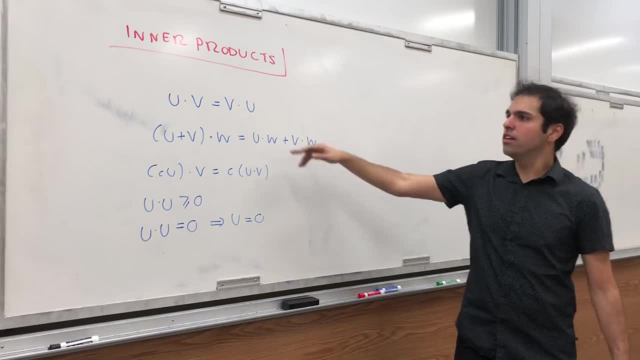 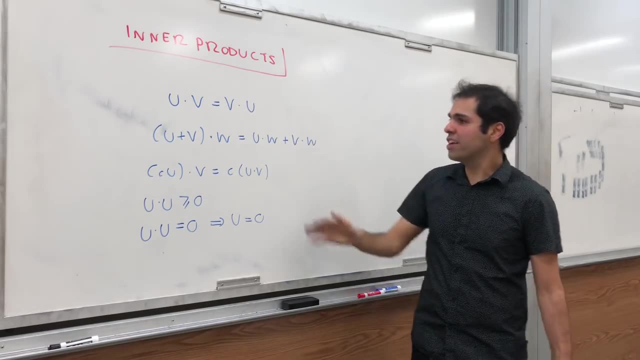 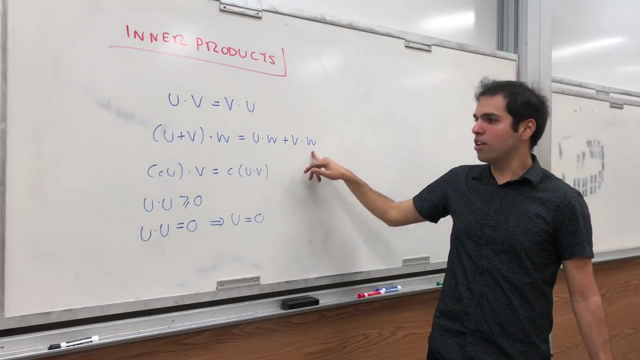 products you use so far they're just those ones Namely u, dot v, is v, dot u, and I'm doing it on real space for complex numbers. You put a bar here, but not today, And you have sort of a distributive property so you can FOIL out dot products And also, if you multiply u by a number, you can just: 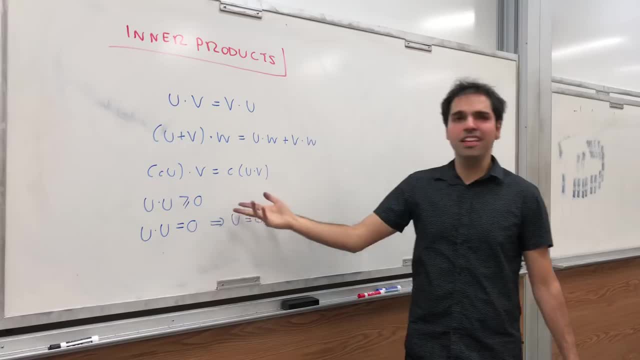 take that number out from the dot product. And, lastly, you just use the fact that if you dot a vector with its center, you can FOIL out a vector with its center. And, lastly, you just use the fact that if you dot a vector with its center, you can FOIL out a vector with its center. you can. 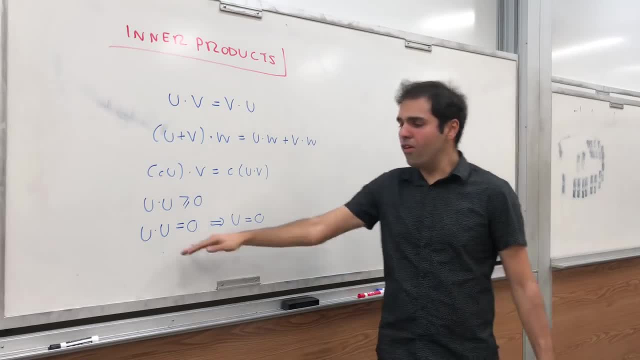 FOIL out a vector with its center. you can FOIL out a vector with its center And if u dot v itself, it's greater or equal to zero. And the only way u dot u is zero is if u itself is a zero vector. 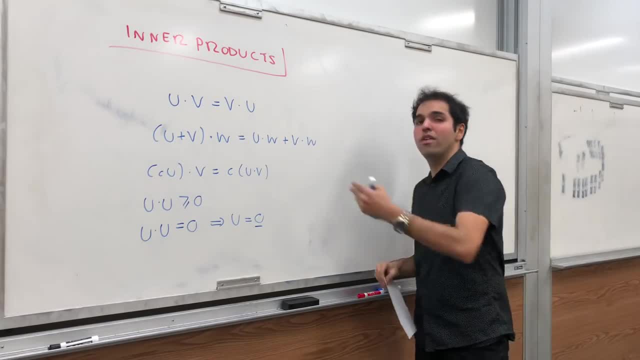 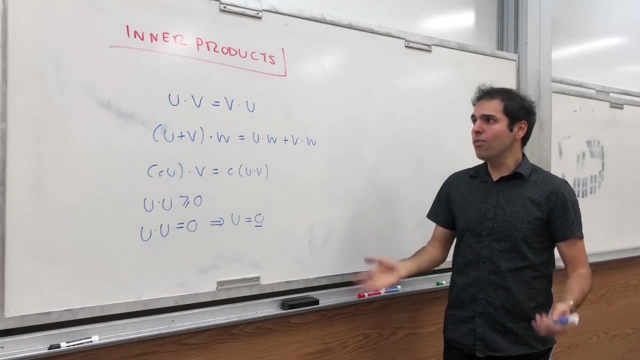 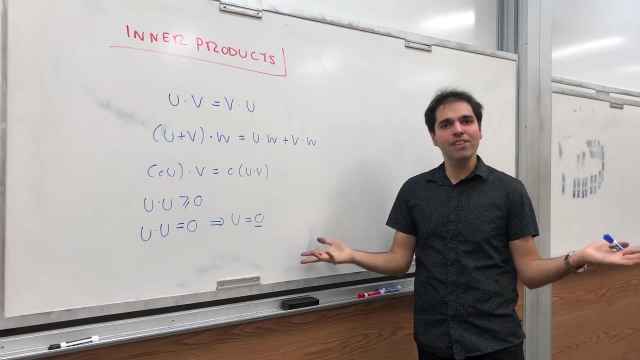 So again, you may not have thought of it this way, but really those are the properties you use. And what is an inner product space? It's just a space with a dot product just satisfying all those properties. In other words, let's forget everything we know about dot product. 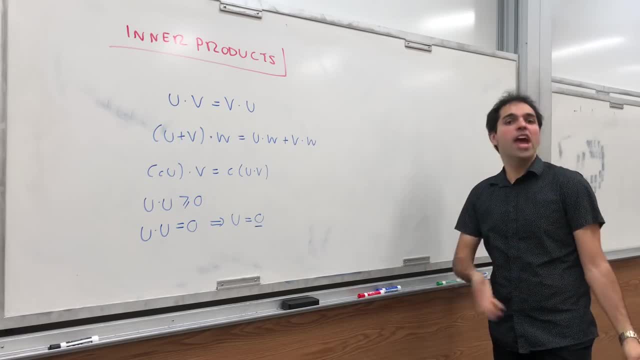 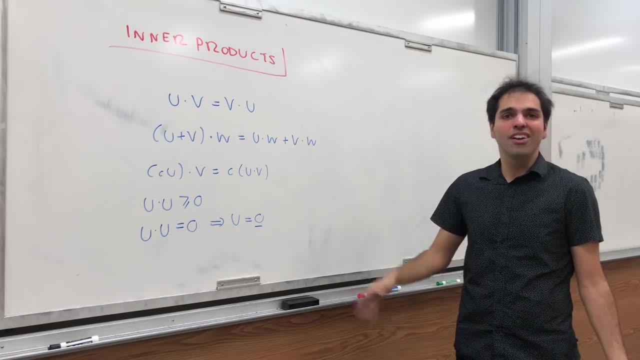 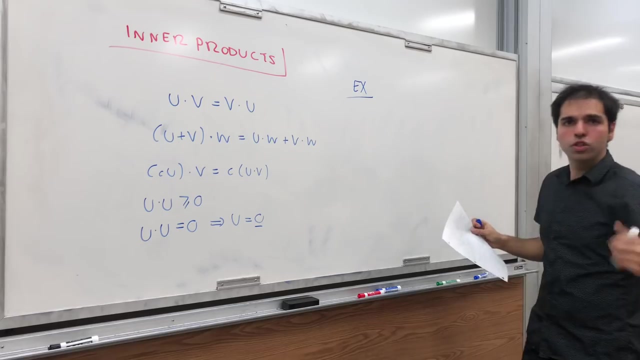 except for those properties. And today I will just give you some examples and I'll just show you that they're not too different. What we've done so far is not too different from what we'll do today. For example, take the space R2,. 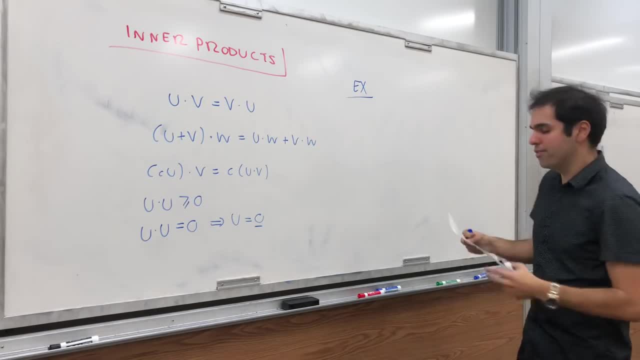 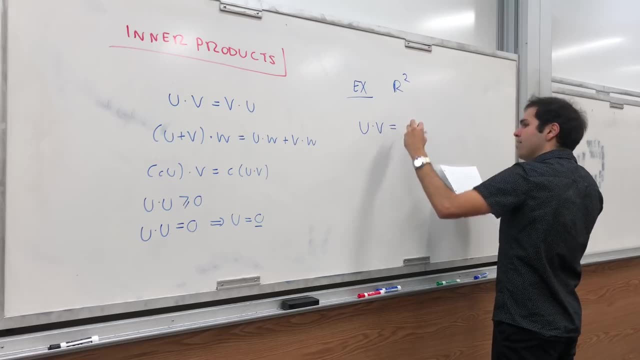 and by space I mean vector space. but that's not the point of today. Take R2, but u dot v. it's simply so. if u is u1, u2, and v is v1, v2,, then u dot v. it's simply the usual dot product. 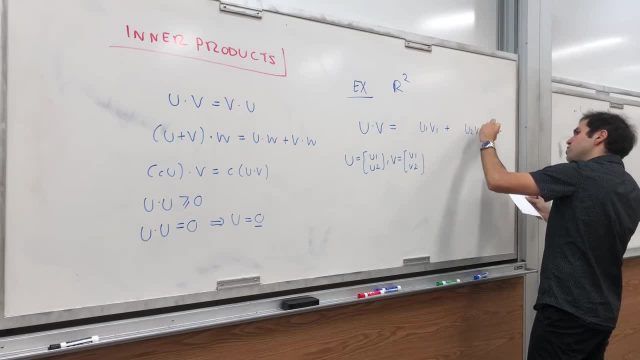 u1, v1, plus u2, v2, except you put extra numbers. so five here, four u1, v1, plus five u2, v2.. In other words, you take the dot product but you sort of wait. 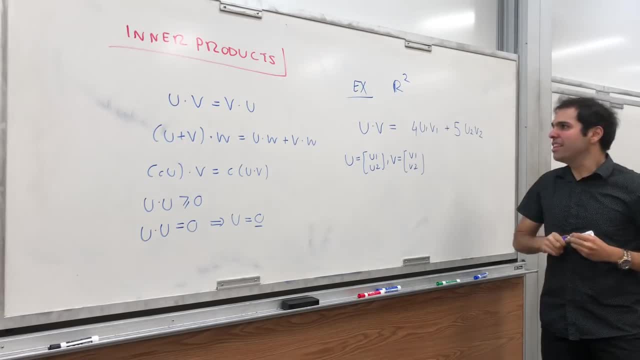 You weigh the weights here a little bit, And that's good if you want to say: well, I really want to emphasize, let's say, the first component and I want to de-emphasize the second component, if you'd like. 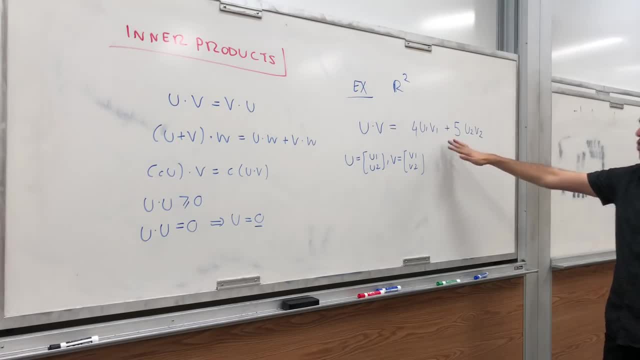 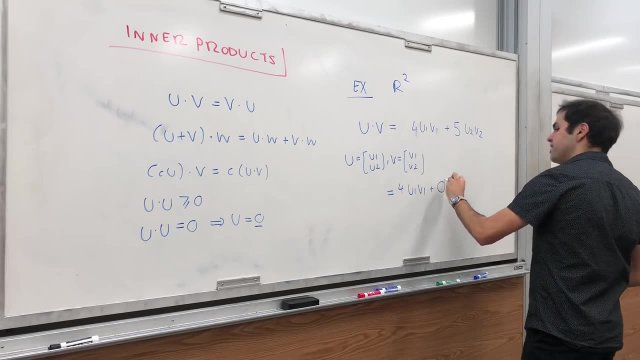 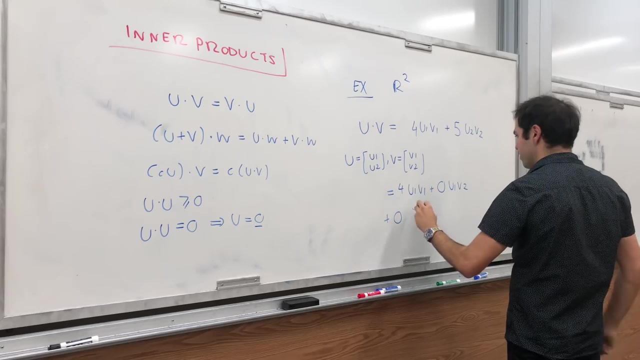 And notice we can actually put this sort of in terms of a matrix, because this is really four u1, v1, plus zero u1, v2, plus zero u1, v2.. U2, v1, plus five u2, v2, I think that's what it is. 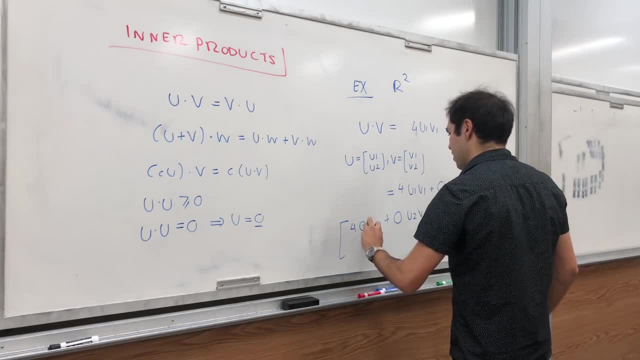 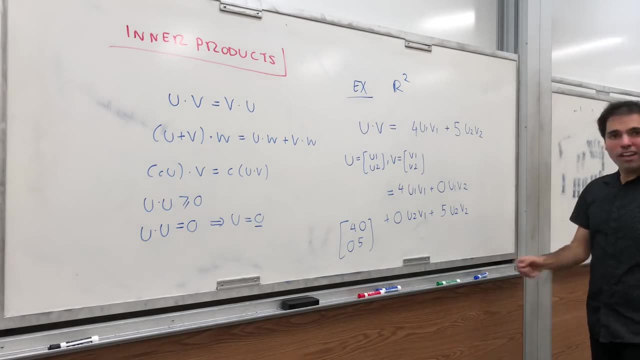 And you can write this as four zero zero, five. And in particular- here's the interesting thing- What is the most general dot product? we can put on this, on R2 or on RN, and it turns out the most general dot product. 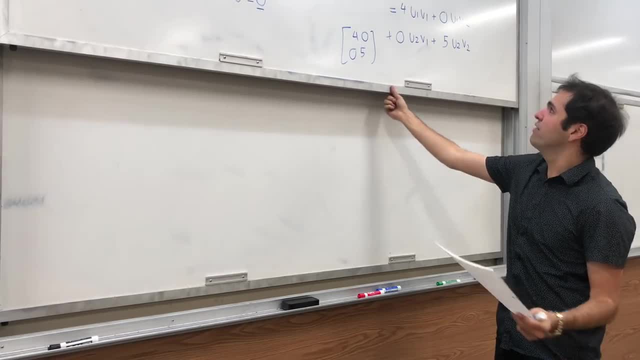 we can put on this on R2 or on RN and it turns out the most general dot product. we can put on this on R2 or on RN and it turns out the most general one you have. so, by the way, you can just write this as u dot v. 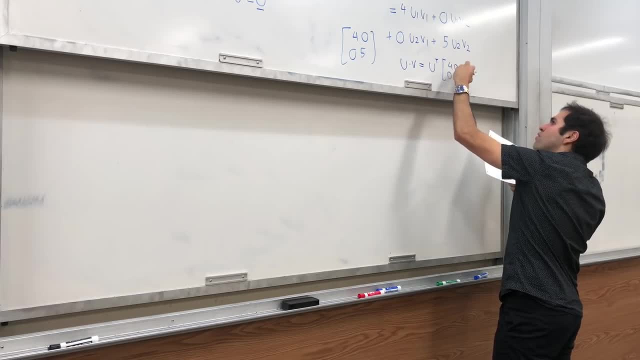 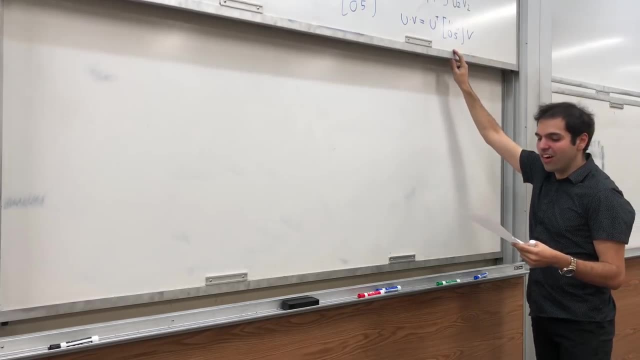 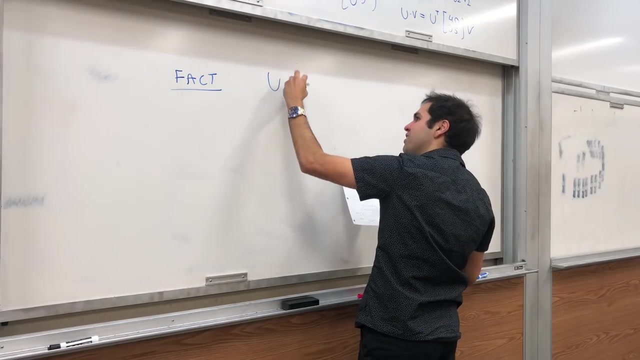 is u transpose four zero zero, five v? The question is: what is the most general form of a dot product on RN? It turns out it's the following fact: The most general dot product you can put on RN is u dot v. is u transpose a v? 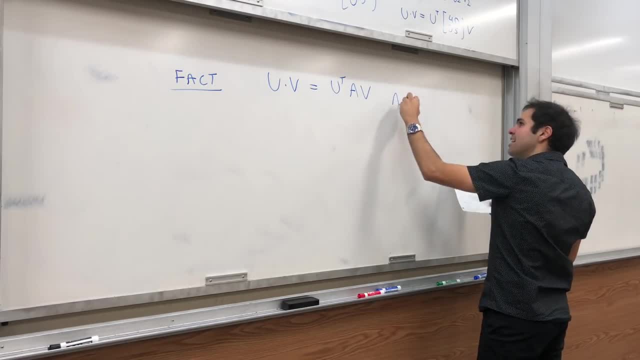 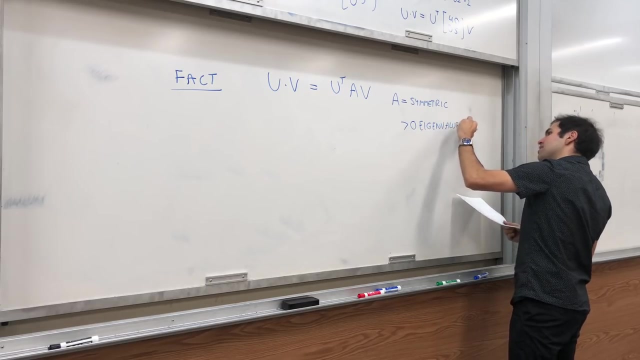 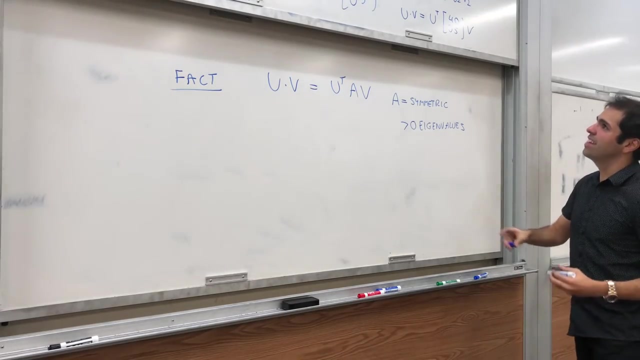 u transpose a, v, where a is a symmetric matrix, matrix that's positive, definite, in other words with only positive eigenvalues. and, by the way, a symmetric matrix is always diagonalizable. so this does make sense and here, for example, yes, we have a symmetric matrix with positive eigenvalues. so just if you're curious, 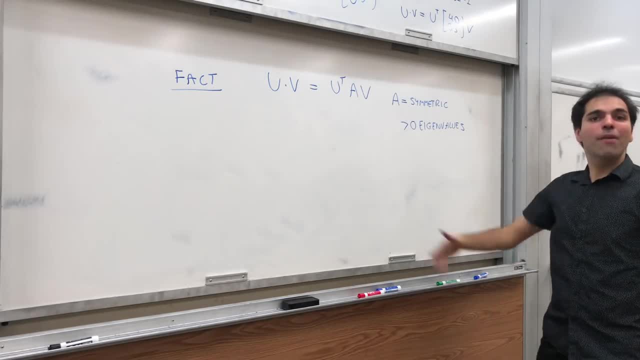 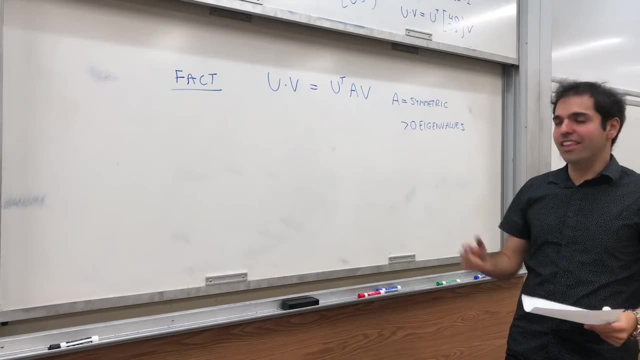 and I think when I teach my more advanced course I might do a proof on this. so it's very neat, okay, so there was one kind of a dot product where you weigh things a little bit. the second kind of dot product is, for example, on the space. 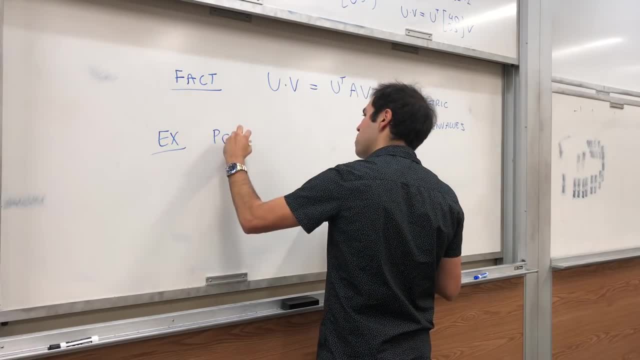 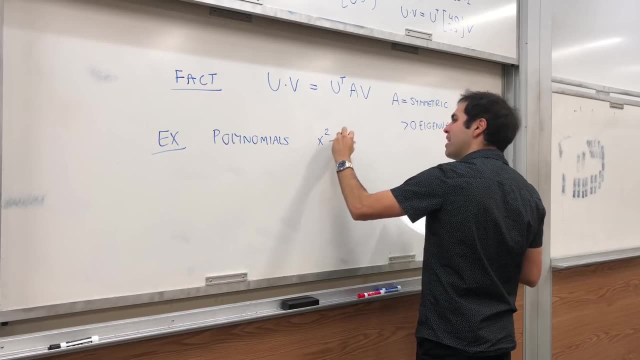 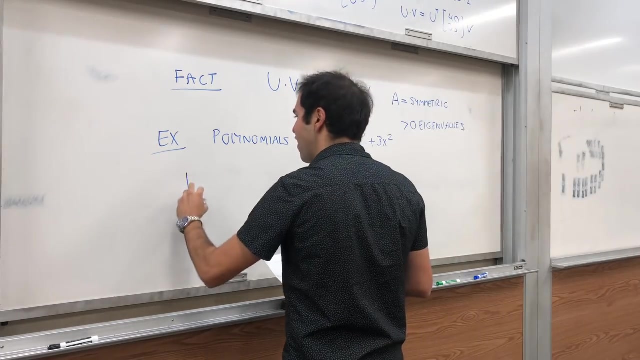 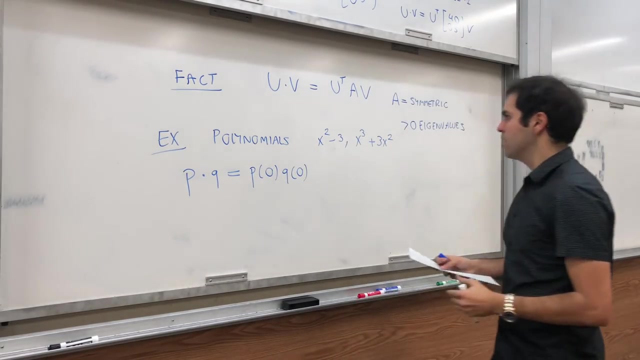 of polynomials. so take polynomials, suppose you know, like a, I don't know- polynomials like x squared minus 3, or x cubed plus 3x squared, etc, etc. then you can just define p dotted with Q to be P of 0, Q of 0. so for example here, x squared minus 3. 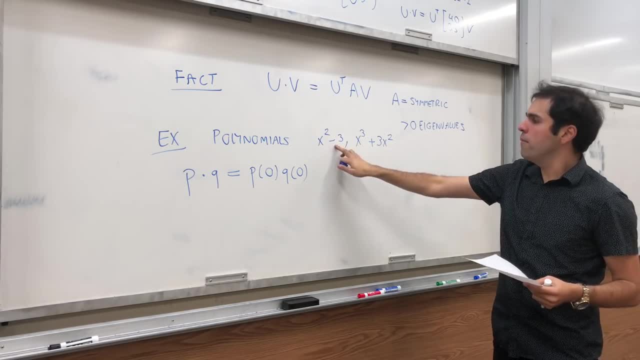 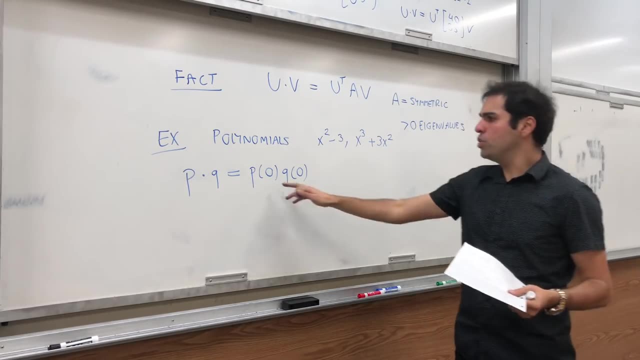 dotted with x. cubed plus 3x squared would be minus 3 times 0, which is 0, and in particular there's nothing special about 0. you can do it at 1, at 2, at any number you want, and in fact you can. 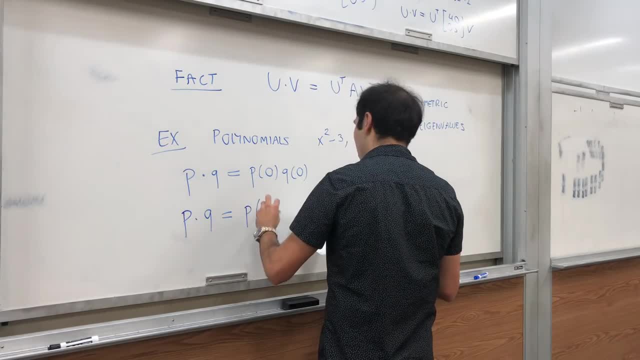 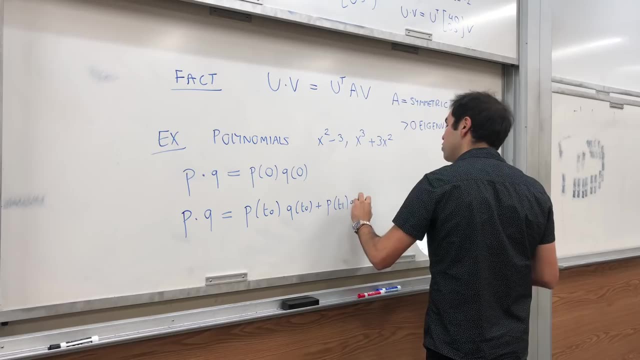 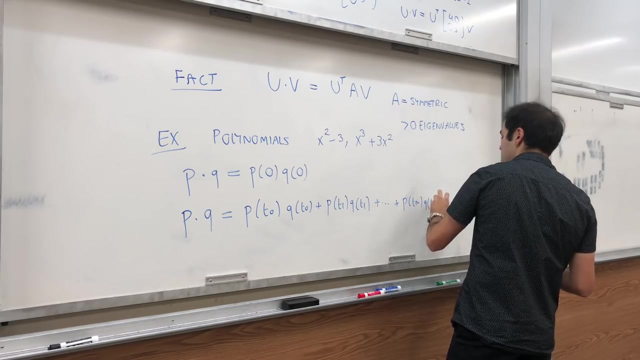 combine this. you can just do P of 1 point t naught, Q of t naught plus p of t 1, Q of t 1 plus dot, dot dot, plus P of T n, Q of T n, in other words, your Sam, what's called? are you sampling your polynomials and then you start to do well on this one. 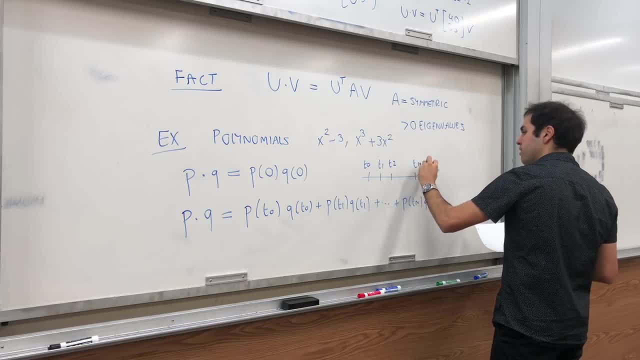 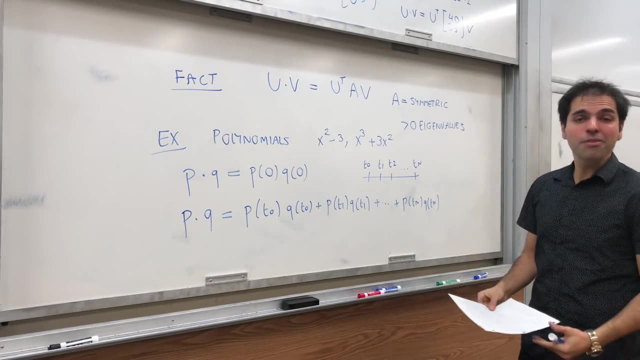 Add some nodes t0 up to tn. If you do that you get another dot product, And I think it's useful. maybe you know, in Riemann integration you use sort of that thing as well. So that's one thing. 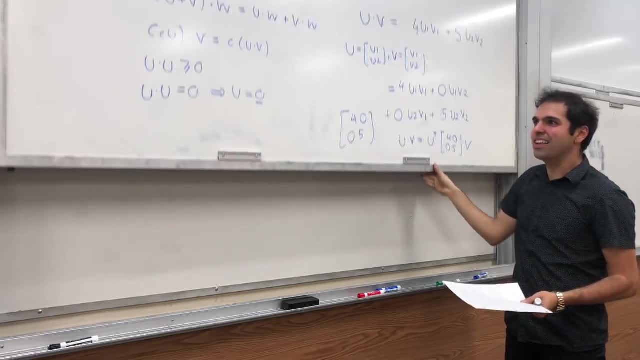 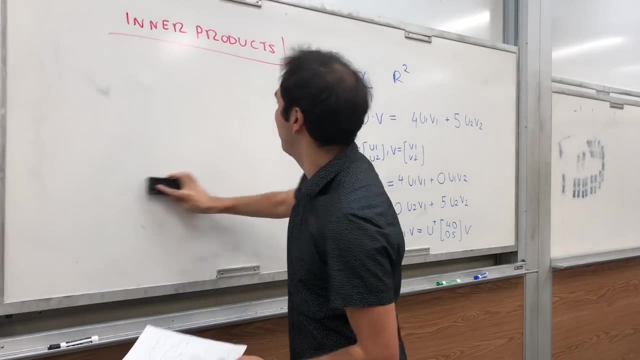 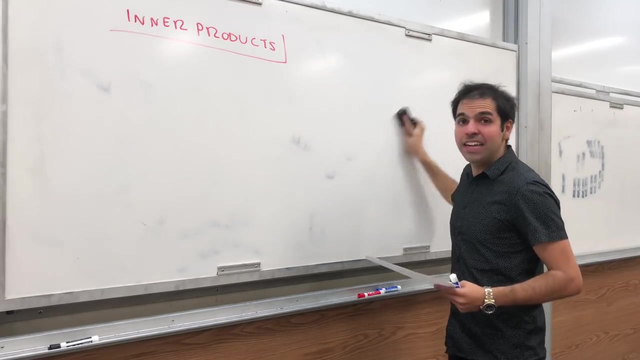 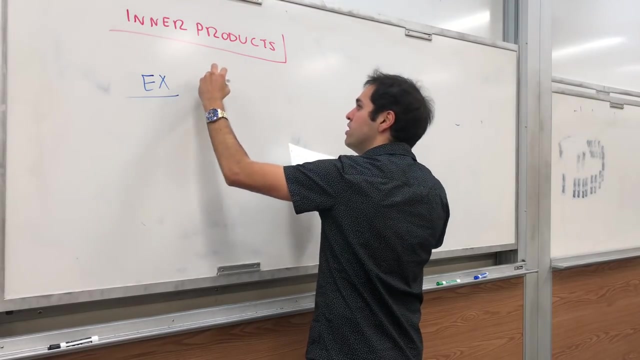 And then the most important example I want to talk about, it's simply continuous functions. So you can take dot products of functions in general, Namely one that looks brand new but that's actually not quite new. So if you have the spaces of continuous functions on a, b, 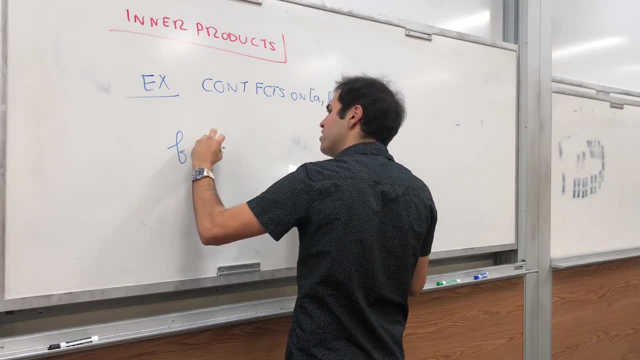 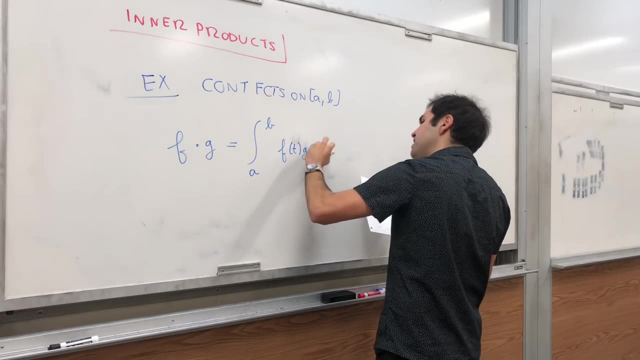 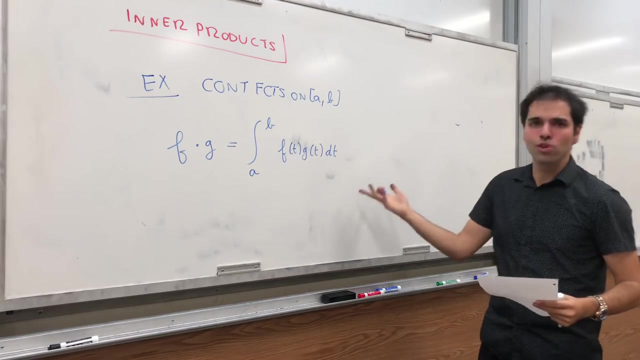 then you can take f dotted with g to simply be the integral from a to b, of f, of t, g, of t, dt. And I remember the first time I saw this I was so surprised. But I'm pleasantly surprised, because how cool is that. 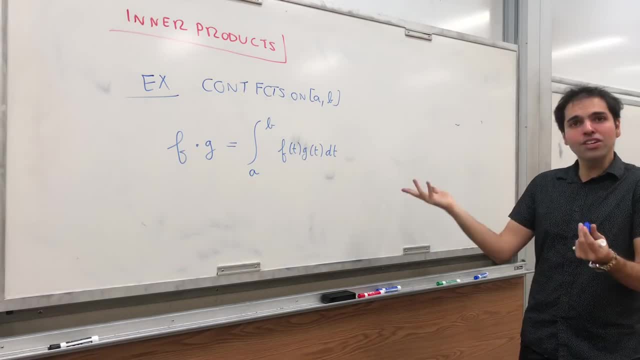 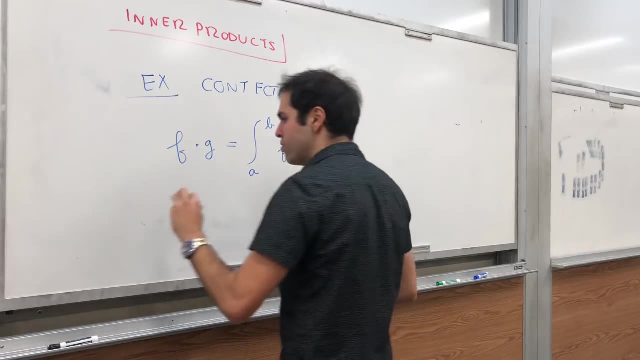 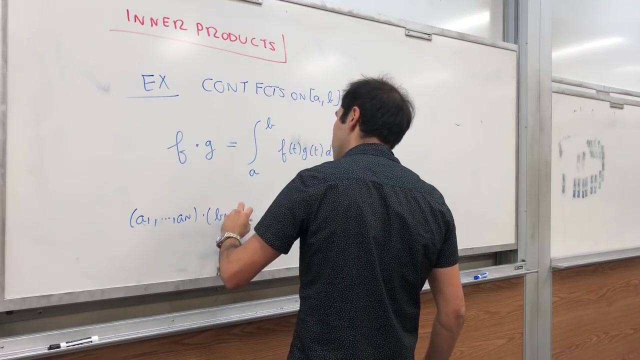 You can take dot products as functions, But I want to show you. it's actually the analog of what you've been doing in Rn. Because what does it mean to take a dot product in Rn? It means a1 up to an, dotted with b1 up to bn. 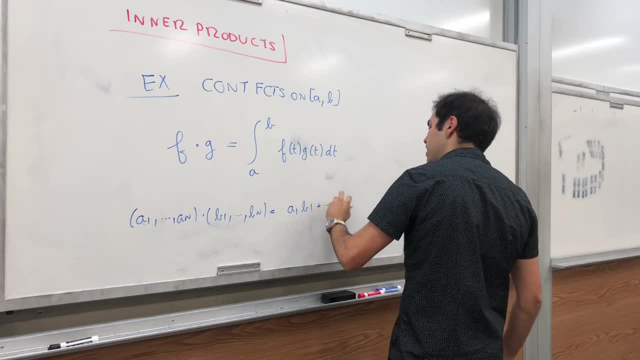 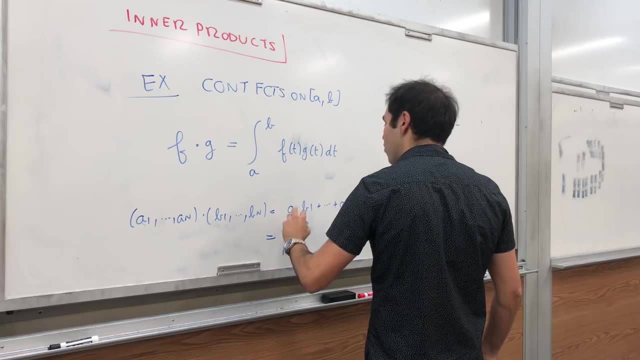 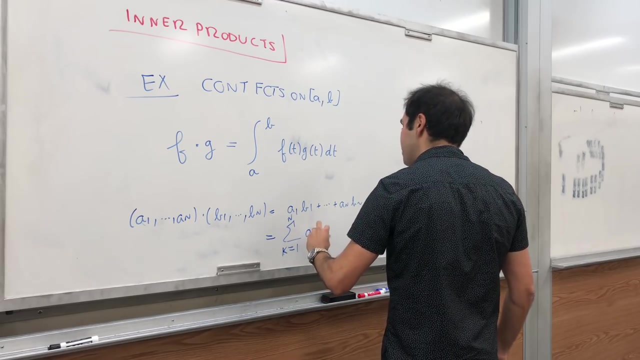 You take, you know, a1b1.. Dot, dot, dot plus an bn, But in terms of summation that's the sum from n from 1.. Sorry, k from 1 to n. n of ak bk. 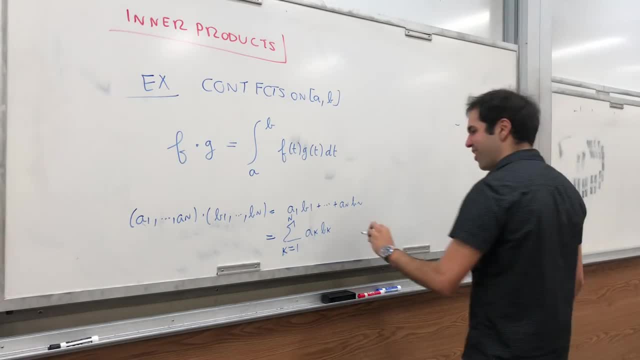 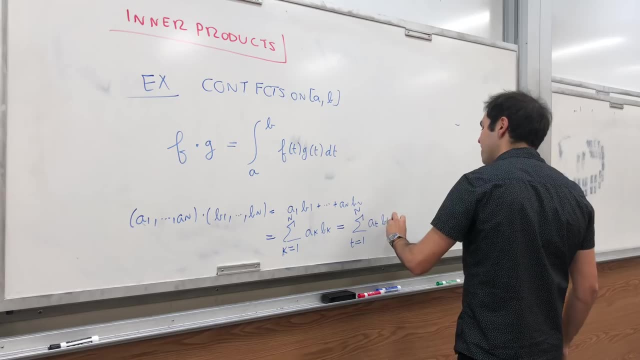 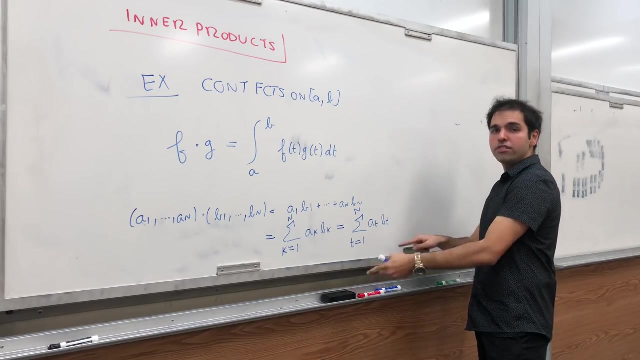 And let me abuse notation a little bit and write it as follows: That's the same as the sum from t, from 1 to n of at bt. So you see, to take dot products, what you're doing: you multiply new vectors and you sum them up. 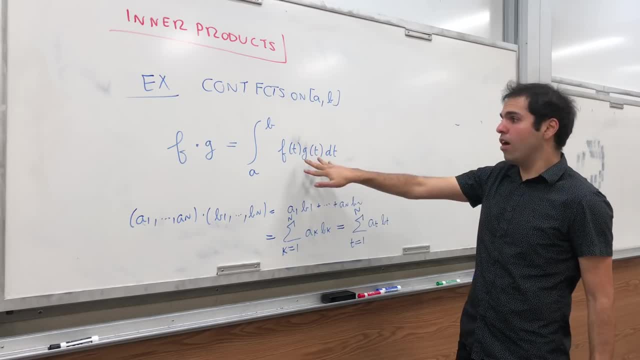 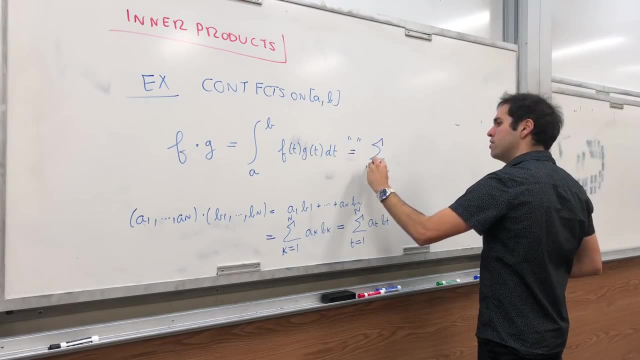 But that's just what an integral is. You multiply those two functions and you sum them up Because, remember, an integral is just a sum. So this is like saying: you sum from a to b, of f, of t, g, of t. 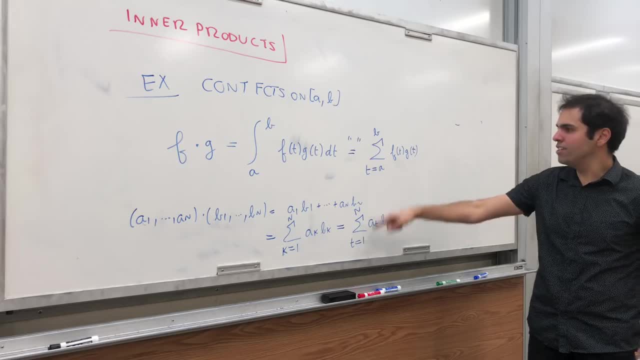 So same thing here. You do. you know f of t times g of t, And you sum, And you sum. So you see, you sum it from 1 to n. That's why it looks like a scary dot product, but it. 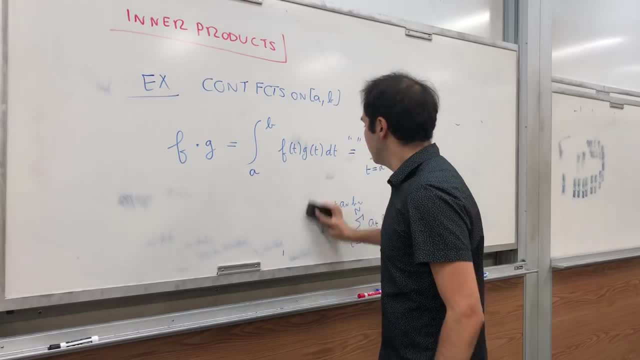 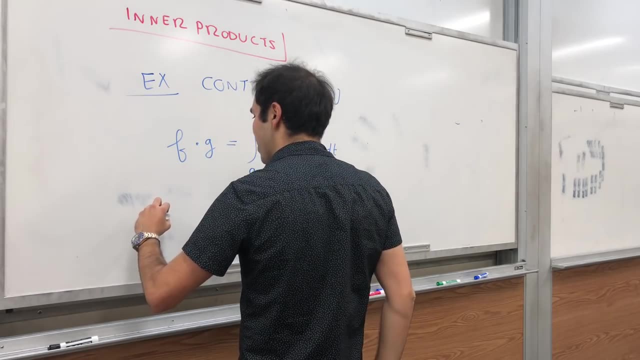 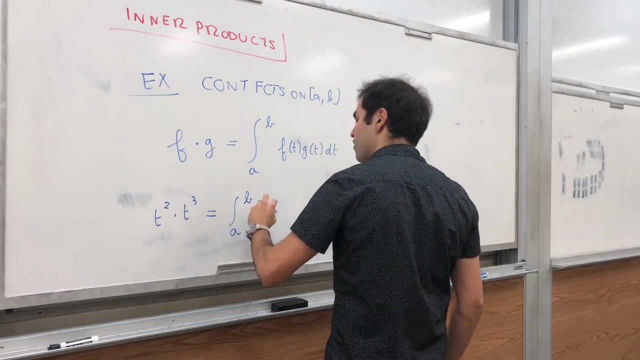 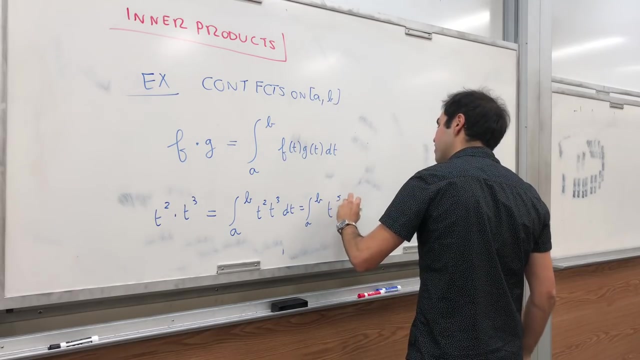 really isn't So. for example, now if you take, I don't know, let's say t squared and you dot it with t cubed, then there's just an integral from a to b of t squared times, t cubed, dt, And that's integral from a to b of t to the fifth dt. And that's, if you. 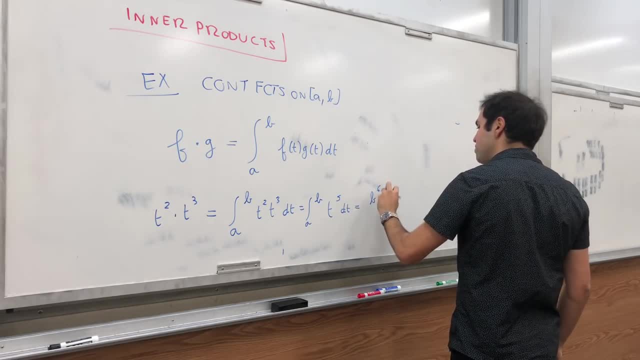 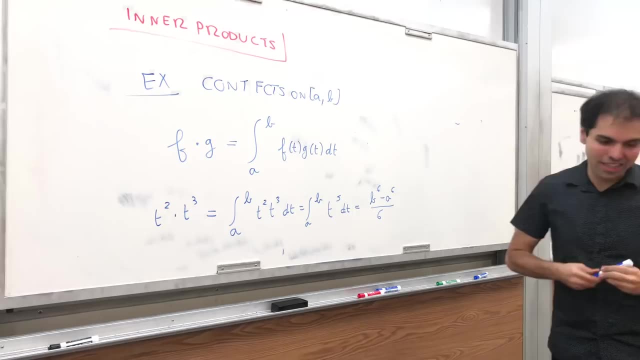 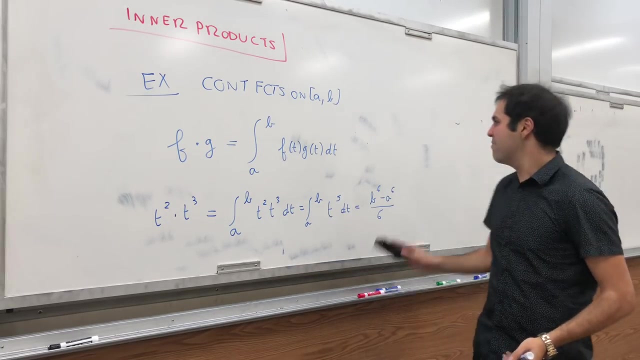 want an antiderivative is 1 sixth, t to the sixth, So b to the sixth minus a to the sixth, over six, And indeed you get a number which is what you expect. And the nice thing is you can everything you've done so far with dot products. you can apply this, So in fact, 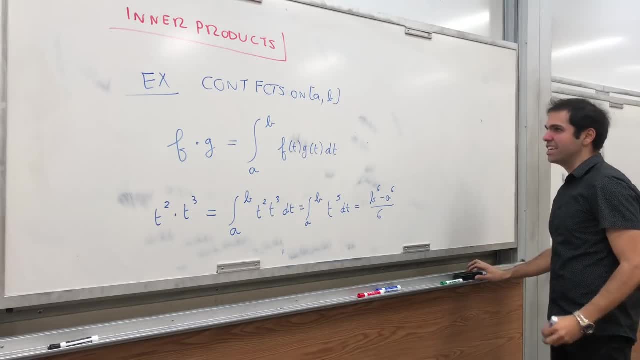 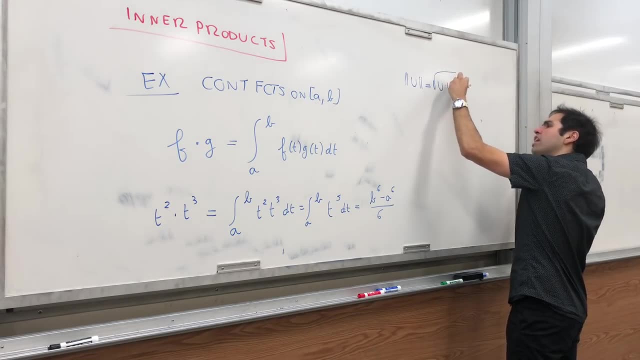 let's use this space as an example For all our techniques. first of all, what is the norm of a vector? Well, it's simply square root of u dotted with u. This is true for dot products in Rn. but the nice thing. 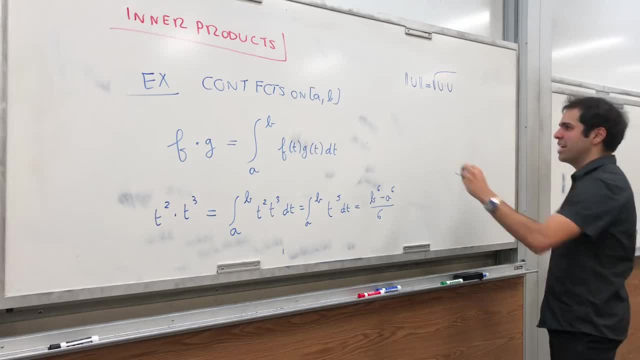 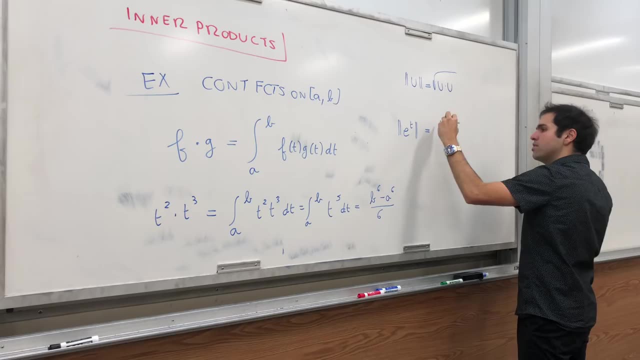 is. this just uses the dot product, so it works in general. So let's, for example, calculate the norm of e to the t with this thing. So it's square root of e to the t, dotted with e to the t. Okay, And that's square root of integral from a to b, e to the t, e to the t, dt. So e, t is. 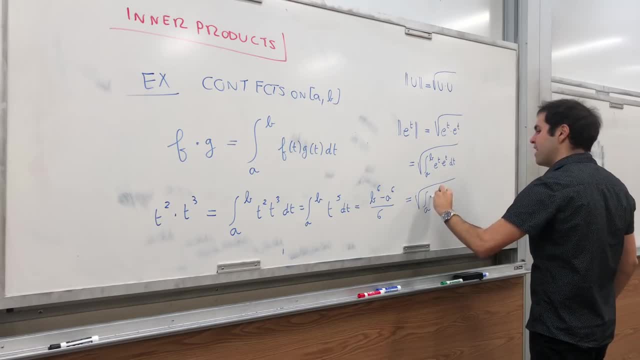 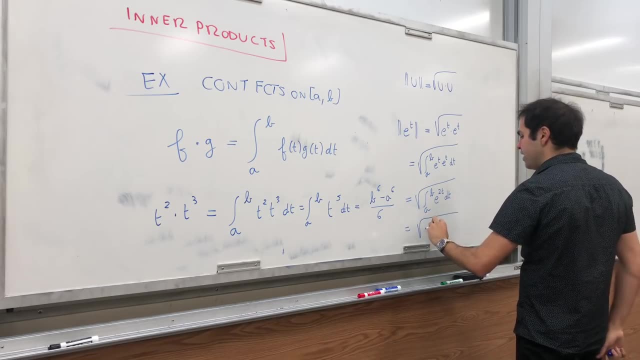 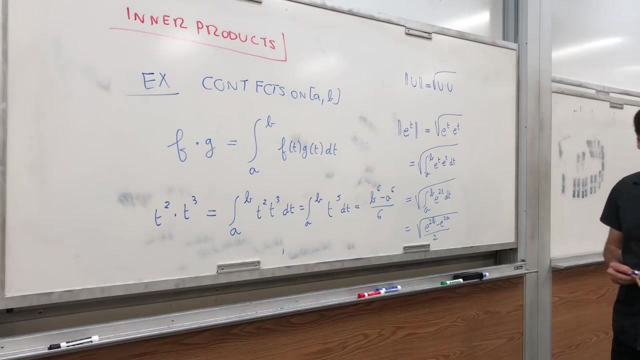 calling home. And that's square root of integral, from a to b, e to the 2t, dt, And that is square root of, you know, e to the 2b minus e to the 2a over 2.. So that is the square root. 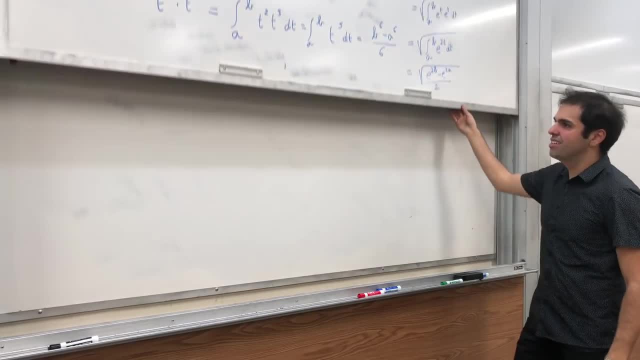 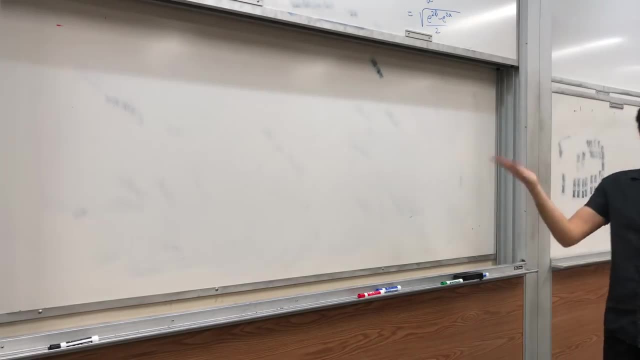 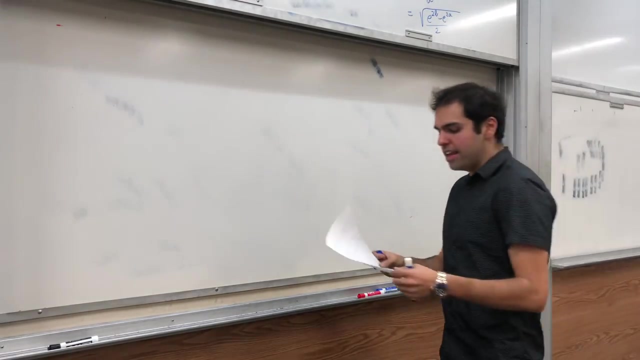 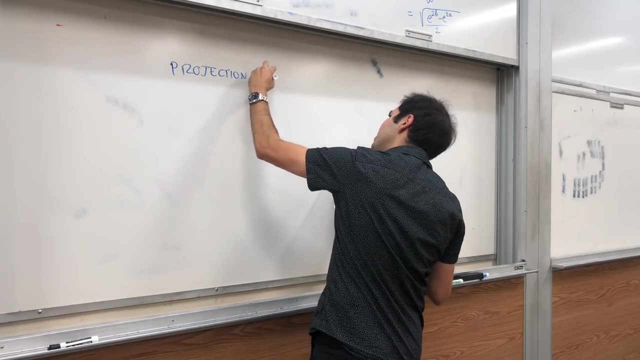 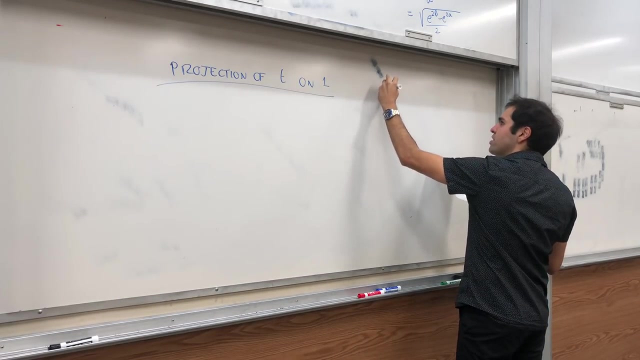 of the function e to the t, And I don't know what that means. you know in practice. And not only that. as I said, everything we've done you can generalize to inner products. So, for example, let's calculate the projection of the function t on the function 1.. Okay, So again we have this function t. 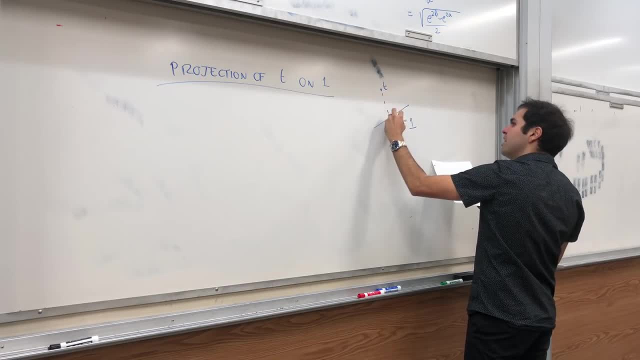 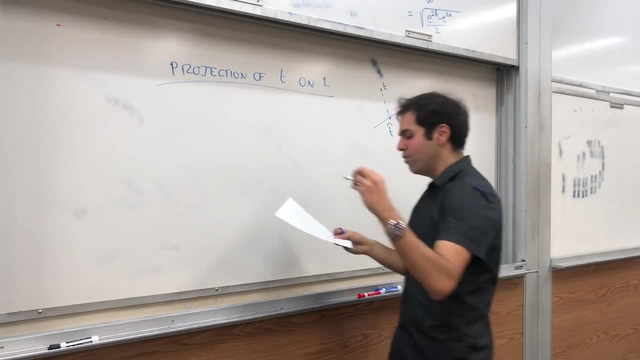 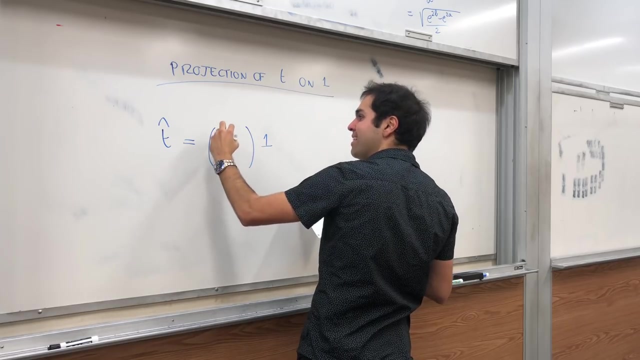 here. This is the function 1.. And we would like to calculate this t hat with the property that t minus t hat is perpendicular to the span of 1.. Well, the formula is exactly the same as before, So it's a multiple of 1.. And the way you do this, you dot t with 1. And 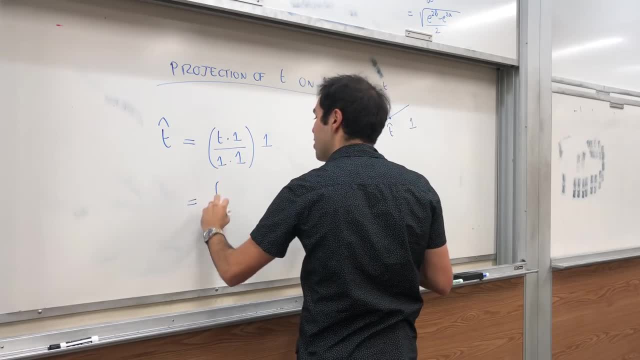 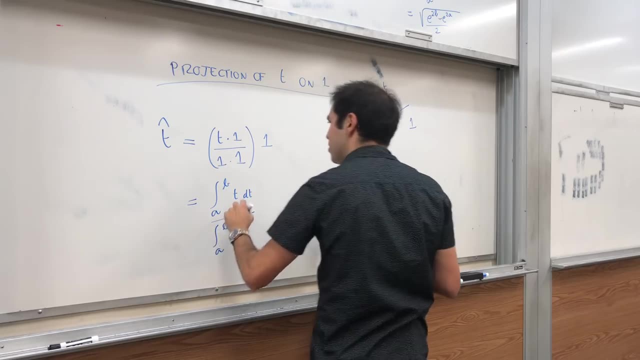 1 is so happy it dots itself. And this time it's just the integral from a to b of t dt over the integral from a to b. So t times 1, which is t, 1 times 1, which is 1. 1 dt. 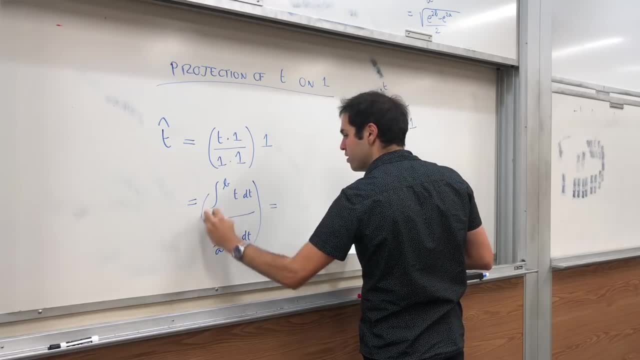 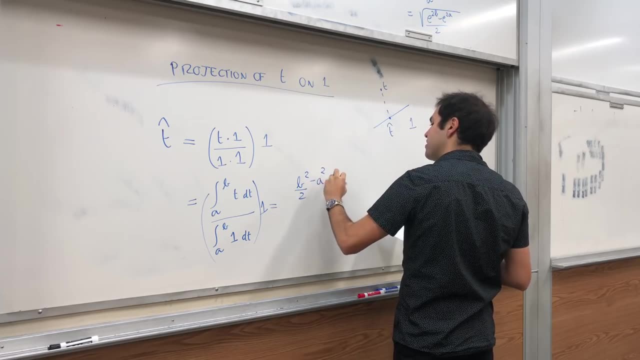 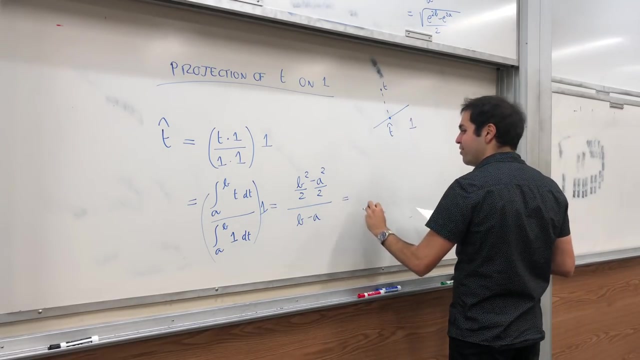 And then antiderivative is t squared over 2.. So, again, this times 1.. So and this becomes just b squared over minus a, b squared over 2 minus a squared over 2 over b minus a times 1, which doesn't affect anything, And you can simplify this a little bit. So that's b minus. 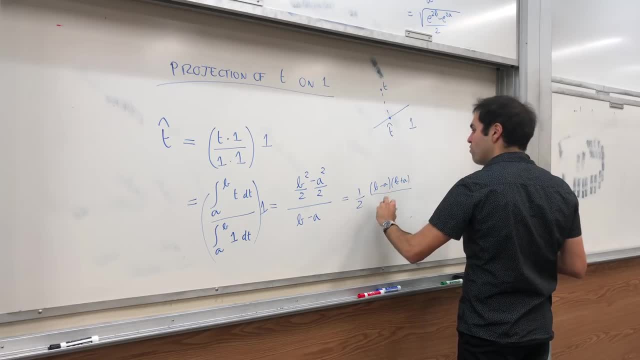 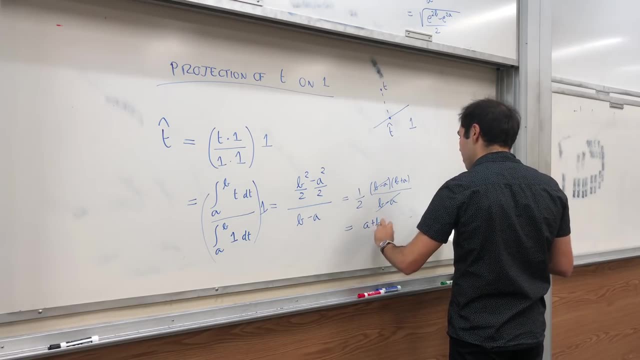 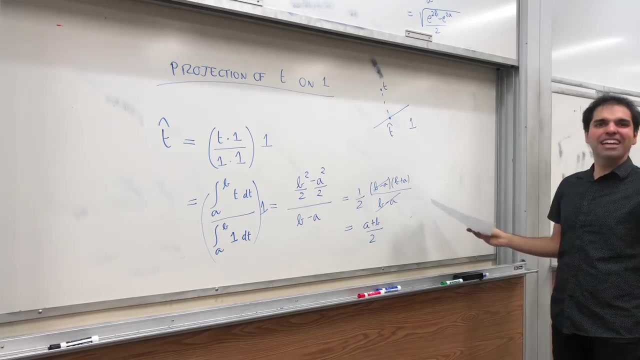 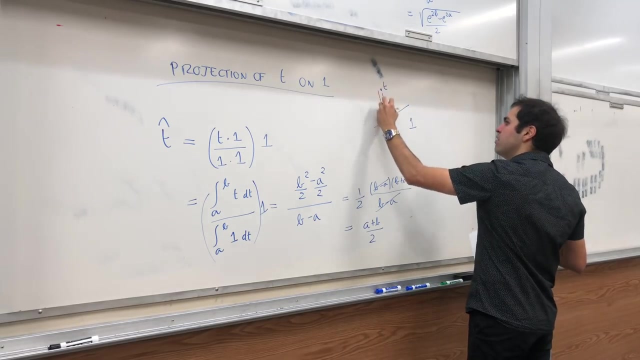 a times b plus a over b minus a, And this cancels out And you get basically a plus b over 2.. Kind of weird. If you project t on the function 1, somehow you get the average of those intervals And in particular, if you want to construct a function that's perpendicular. 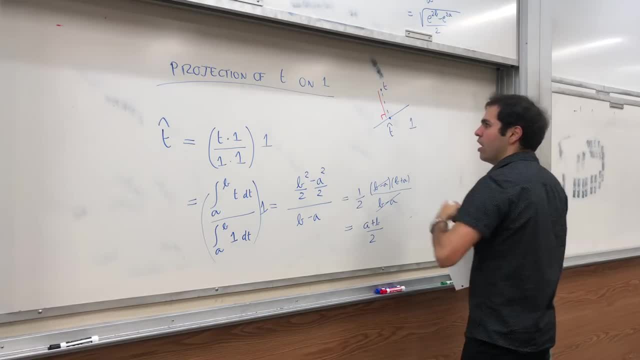 to 1 in this inner product. you just do t minus a squared over 2. And you get a function that's perpendicular to 1 in this inner product. You just do t minus a squared over 2. And you get a function that's perpendicular to 1 in this inner product. You just do t minus. 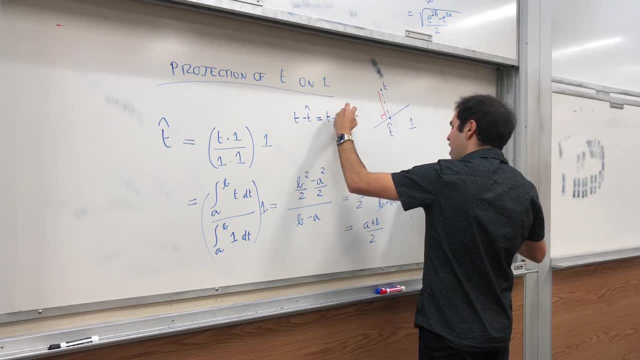 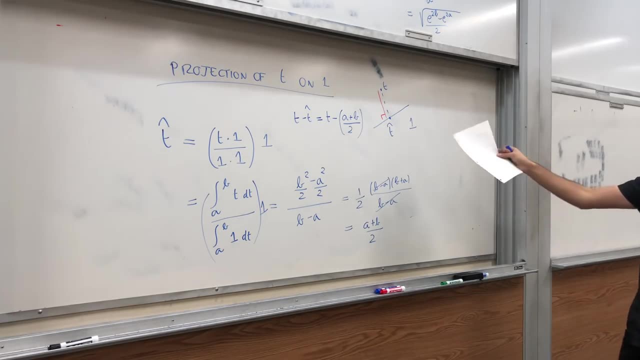 t hat And which becomes just t minus into minus a, minus b over 2.. And indeed, if you dot this with the function 1, you should get 0.. So, yeah, you should get the b squared minus b squared over 2.. Yeah, All right. And in fact, let me check this. I don't believe it. 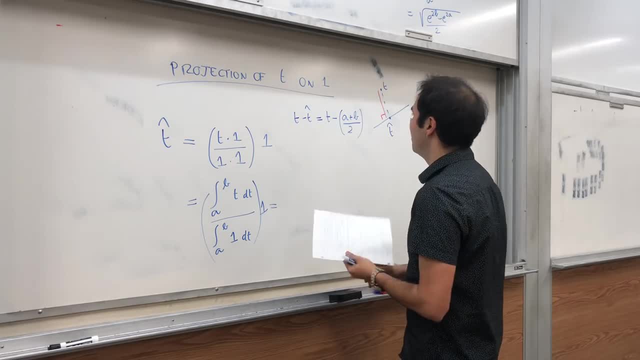 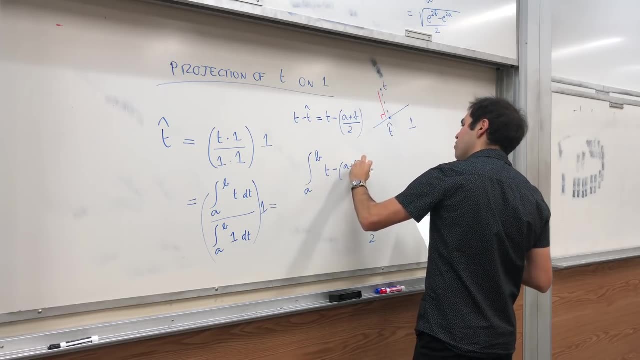 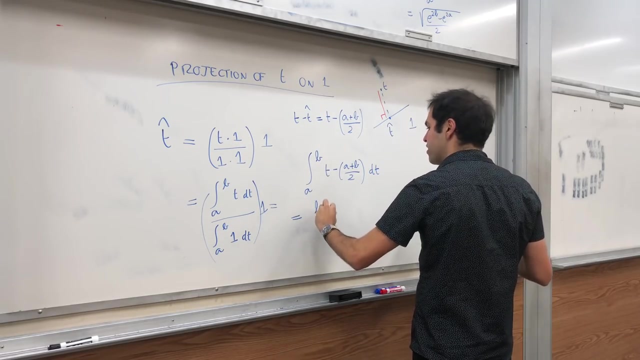 But it should be true. Let me see If you take this. so if you take integral from a to b of t minus a plus b over 2, and you dot it with the function 1, you get this thing which becomes so b squared minus a. 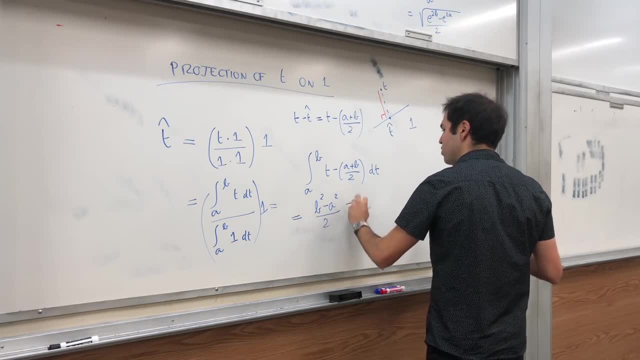 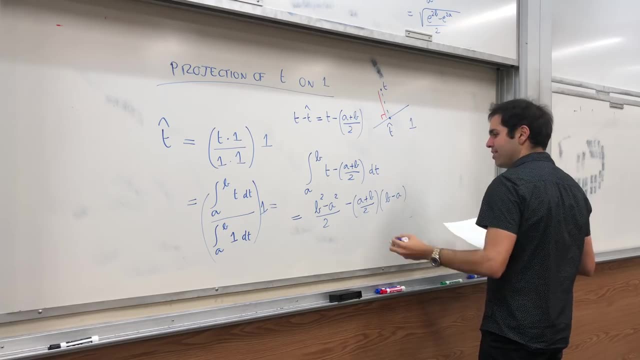 squared over 2 minus. so this is a constant a plus b over 2 times b minus a. OK, This does make sense. So you get b squared minus a squared over 2. So you get b squared minus a squared over. 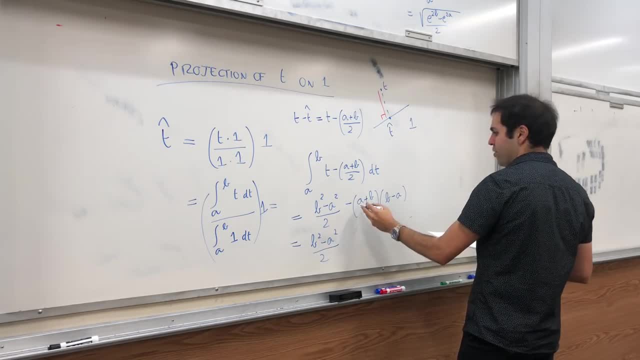 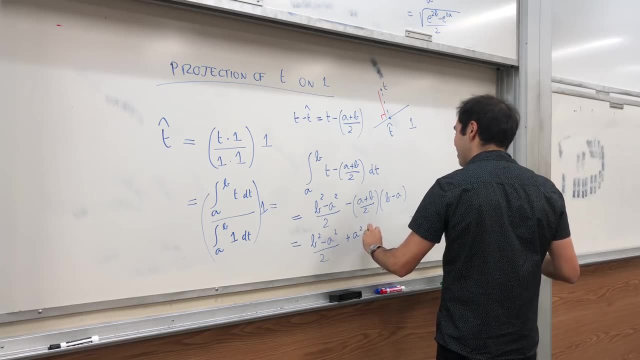 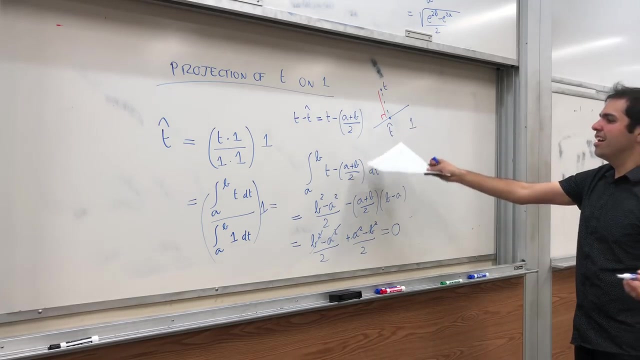 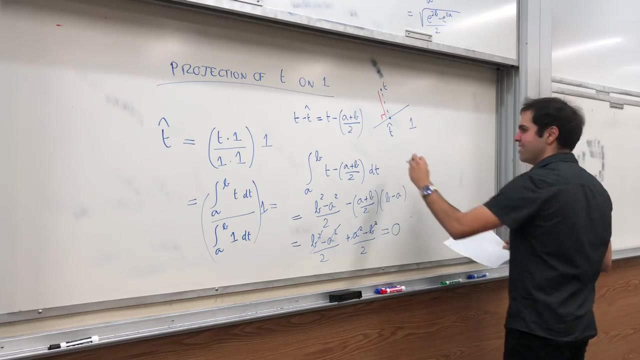 2. And then so basically this becomes a plus b times a minus b, So plus a squared minus b squared over 2.. And then this does give you 0.. So in particular this vector t minus a plus b over 2, and the vector 1, they are perpendicular by this property. So 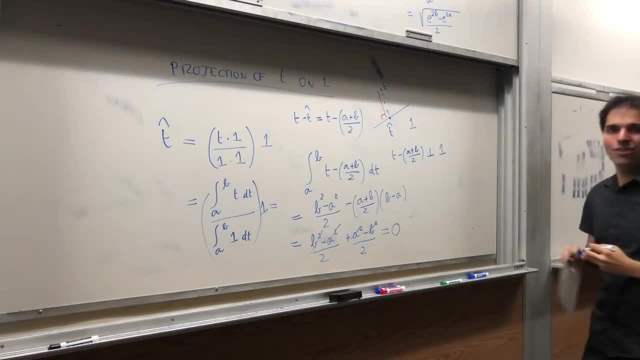 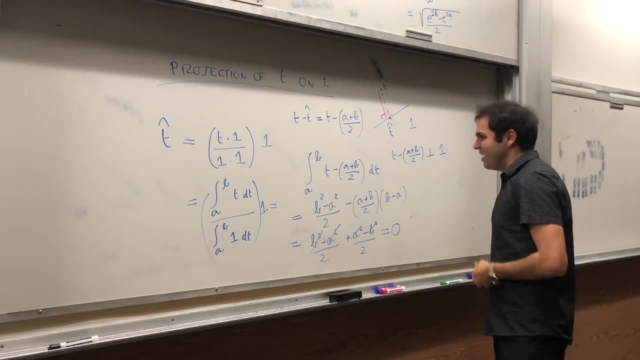 minus b over 2 is in fact perpendicular to 0.. OK, So this is a function 1.. So how nice is this? And, yes, I guess time to stop. That's what the light is telling me, And also you can do other fun stuff with that. 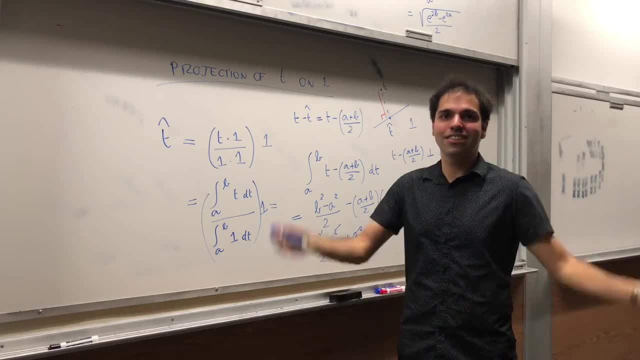 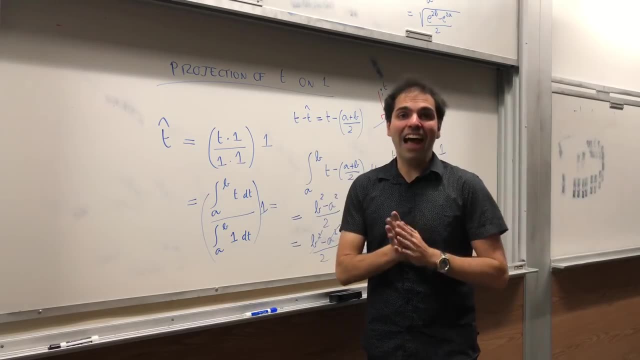 For example, you can apply the Gram-Schmidt process to functions, But that's the point of another video where I will construct the Legendre polynomials. All right, I hope you liked this inner product adventure. If you want to see more math, please make sure to subscribe to my YouTube channel. And I'll see you in the next video. Thank you very much. 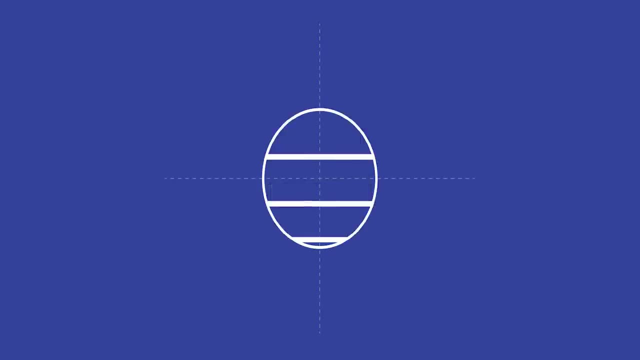 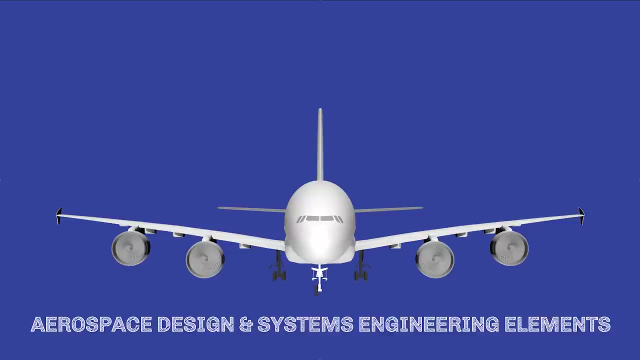 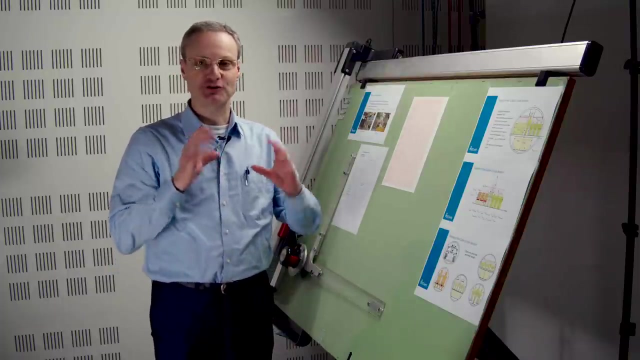 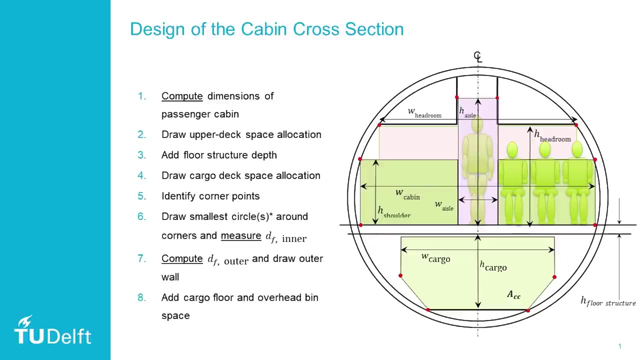 Good morning, good afternoon or good evening whenever you watch this video. Today we're going to make a drawing of the cross-section of the fuselage. We have a 9-8-9 step procedure to follow. This can be found in the slides and this is the procedure we're going to follow. 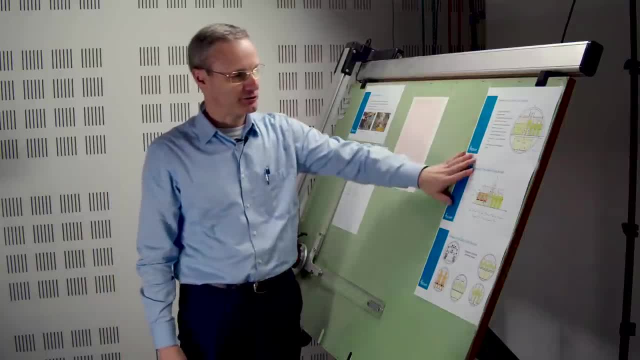 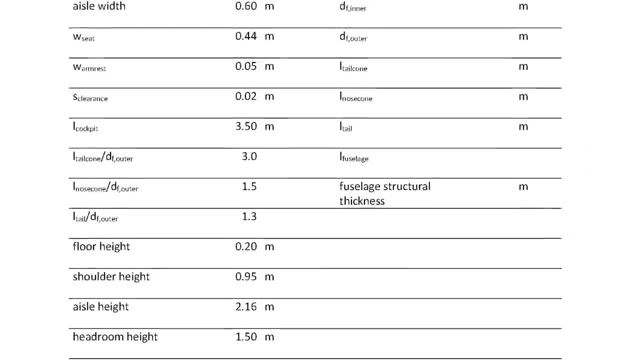 We have a setup here where we have all the necessary slides made available. We have the data sheet, the aircraft design data sheet, and we have some data given and some of the data we need to calculate based on the work we're going to do Here. we have the first sheet of graph paper. 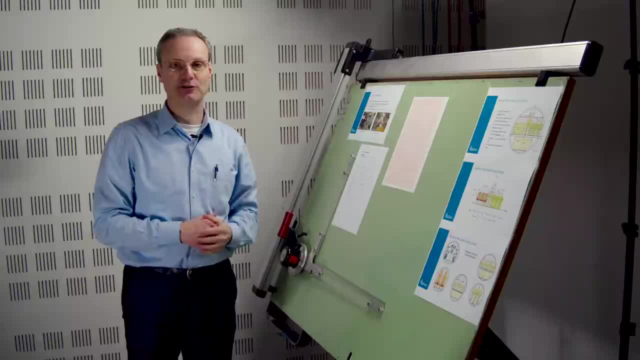 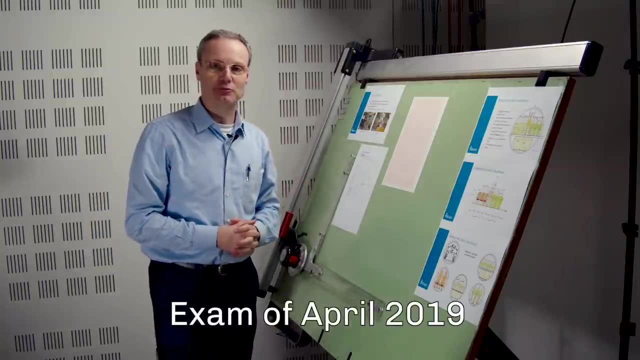 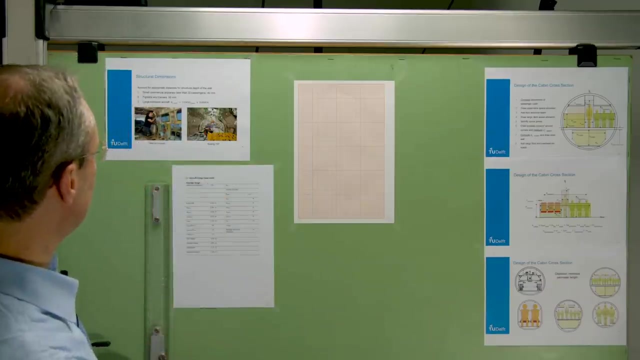 A4 graph paper and here's where we're going to draw the cross-section of the fuselage. The example I will be using today is from the exam of April 2019.. So you can look it back: April 2019.. This is the data we have been given. It's an aircraft for 105 passengers. We have some. 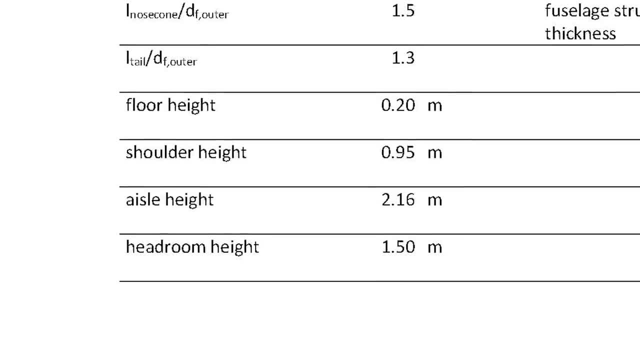 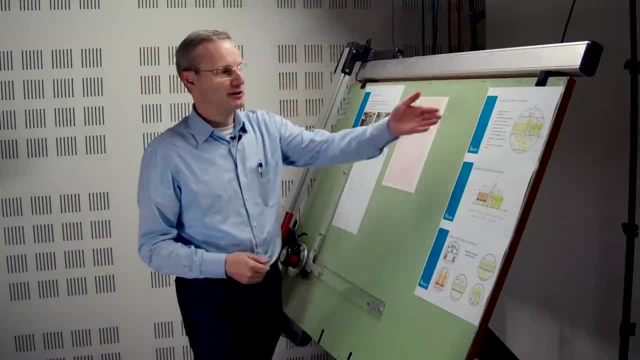 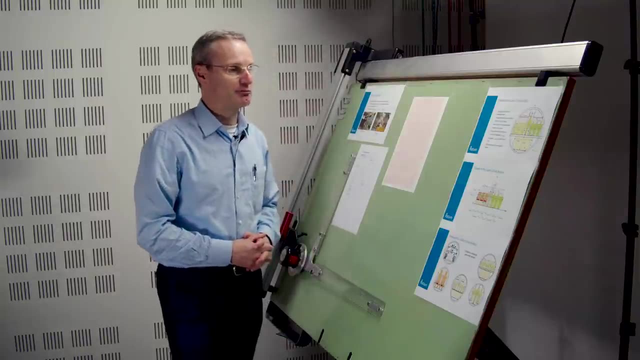 cabin data given so you don't need to calculate that in this case. but we have been given that as a starting point And we need to make a start and then basically try to follow this procedure. Step one says: compute the dimensions of the passenger cabin. For the dimension of the passenger cabin: 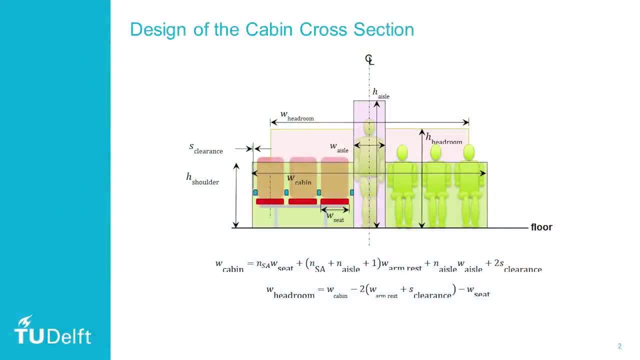 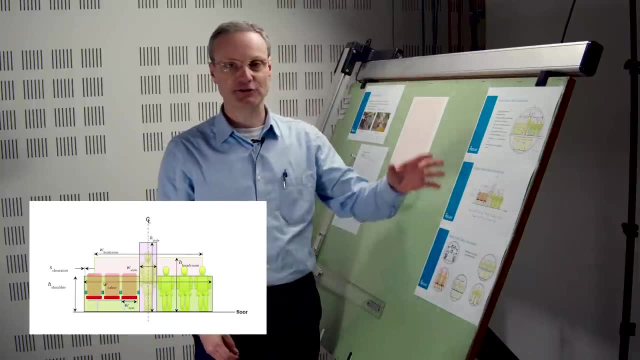 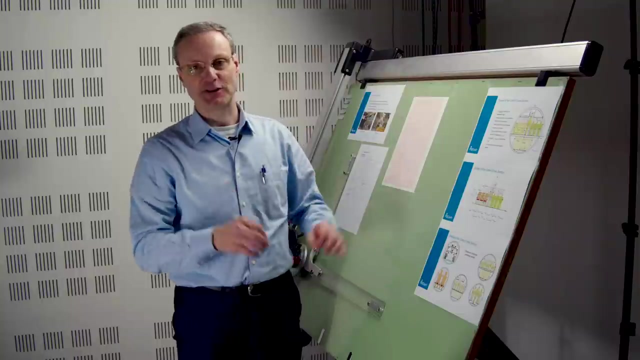 we look at this slide and here we see all the elements we need to put in there. We start by drawing a floor, and then we place the seats, we place the aisles, we replace the headroom, replace the clearances, and with that we can just find the dimensions. After that we're going to.